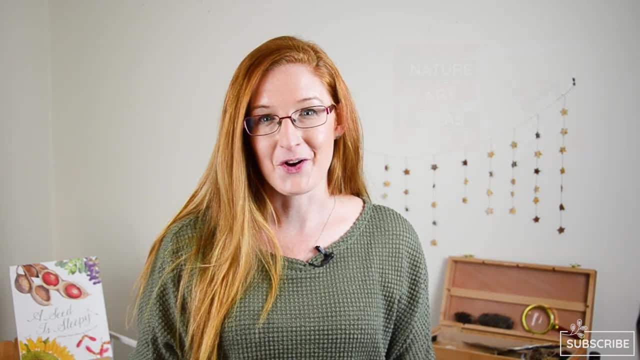 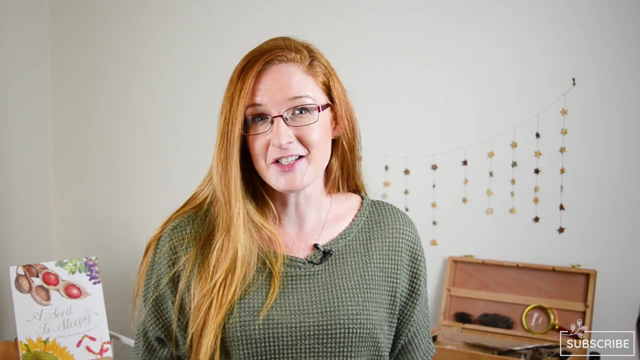 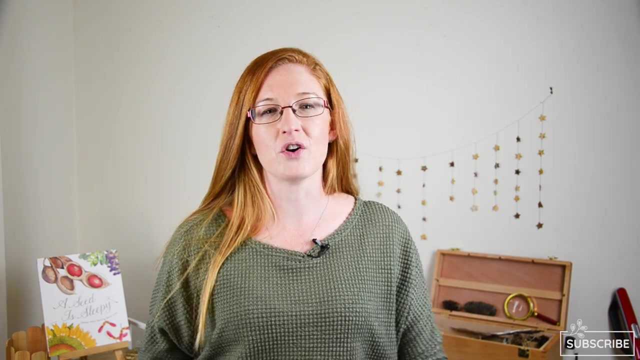 and see that here. If you didn't watch my last video, you may be wondering what's the difference between nature art and nature craft activities? and that's a valid question, because we often use the two interchangeably. Essentially, art is more unstructured and open-ended, while craft usually. 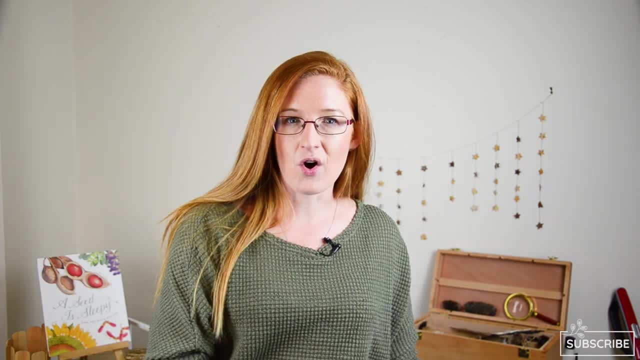 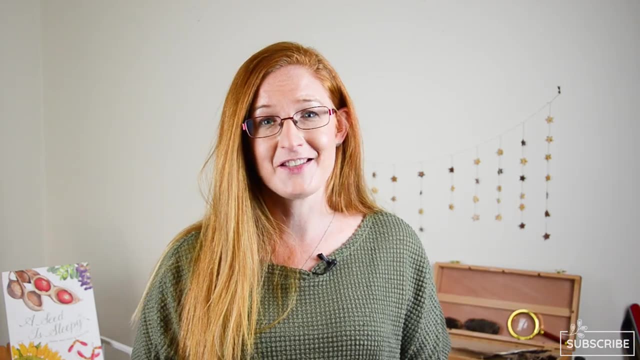 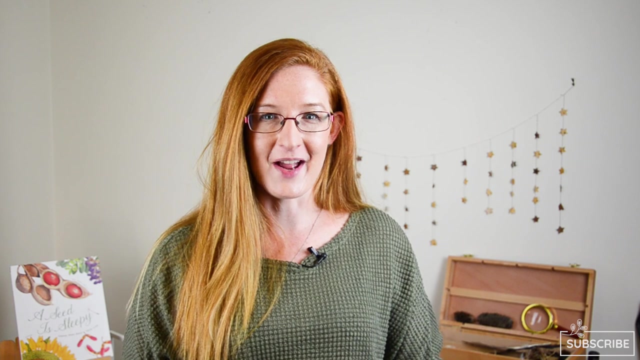 involves a creative process, So if you're interested in learning more about nature, you can head over to this video for those lovely ideas. I'll add the link to the description below. Number one: nature crowns. Children love producing items with their hands and if they get to wear it. 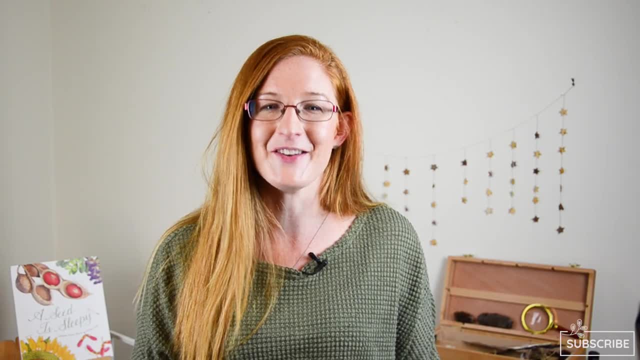 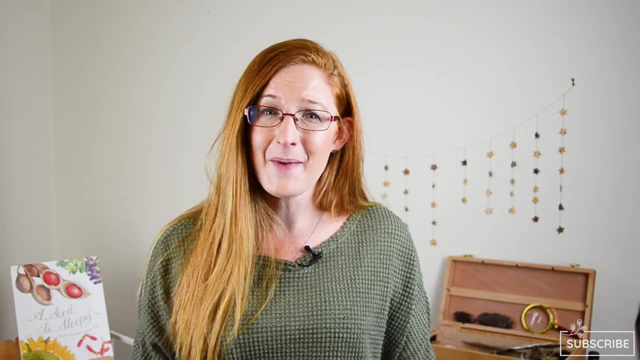 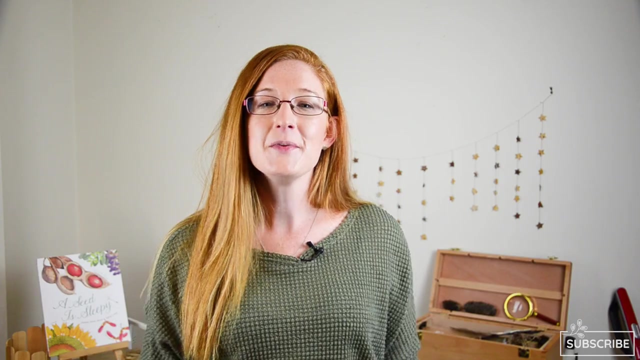 they're even more invested in creating something that suits their unique style. After they're made, children tend to use them as props in play too, But what I really love about nature crowns is that they are always beautiful, no matter the level of complexity or simplicity. Number two is butterfly nature craft. I was lucky. 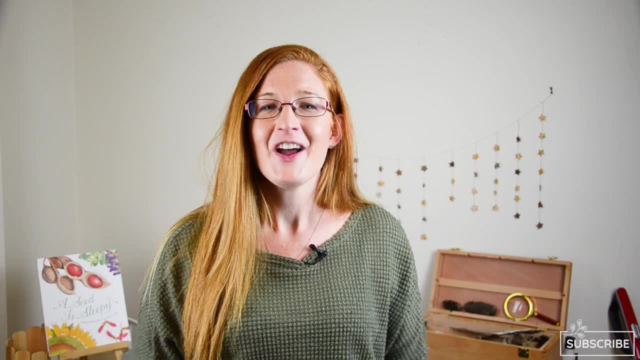 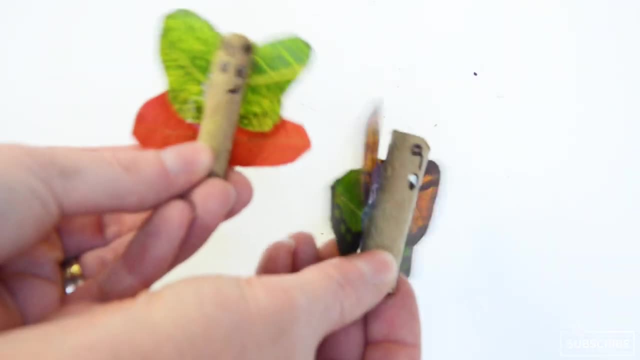 enough to get the creative gene in my family, and I was inspired to make this nature butterfly after I visualized it in my head one day. I made one first and when my daughter saw it they were so excited So I helped them to make their own If your child has an interest in butterflies. 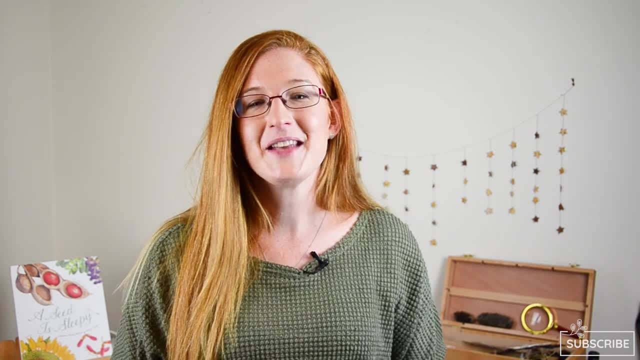 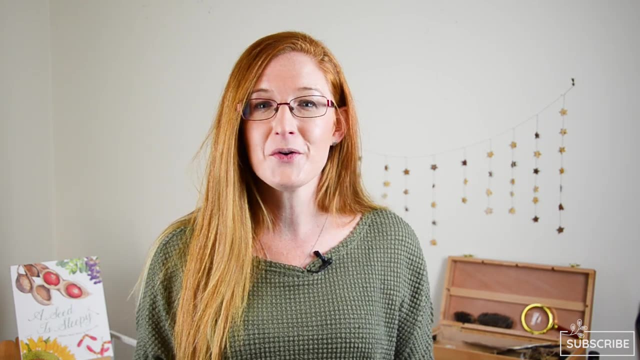 this craft will enchant them. You will need a glue gun, so be sure to take that little bit of plastic off when you retire it to the compost or give it back to the earth. If you're curious how we store our nature crafts, you might like to watch this video after you finish this one. 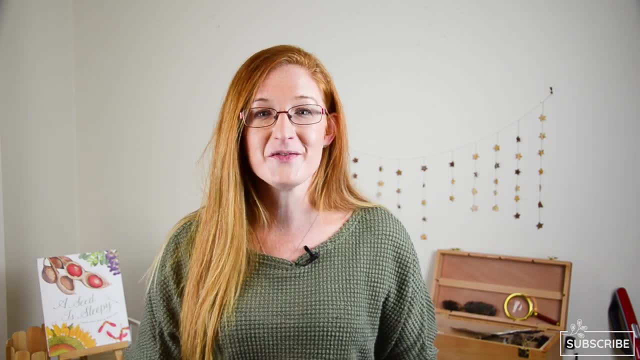 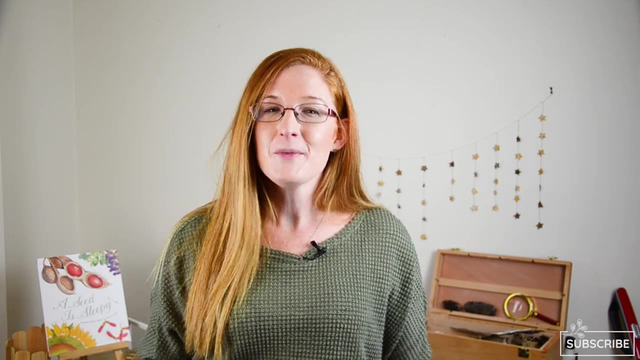 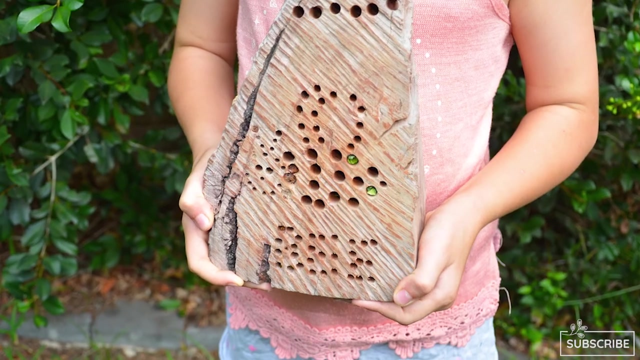 Number three: bug hotel. Tap into your child's affection for bugs by teaching them all about the many creatures that help our local gardens and our greater ecosystems. You may also like to encourage their interest by making this bug hotel. It's super simple to build and it will add some artistic flair to your backyard. 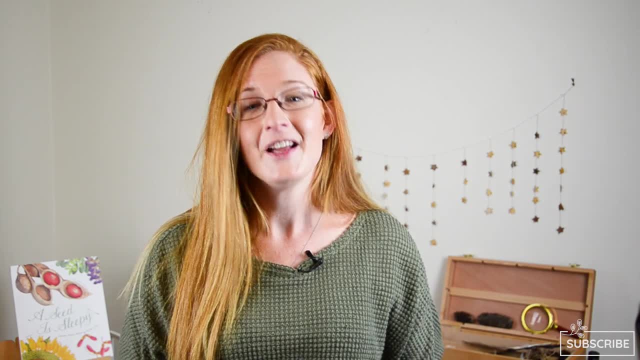 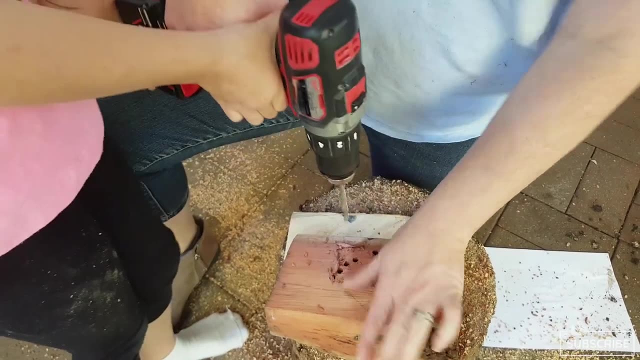 You might like them so much that you want to produce more than one for your garden. The good news is it costs almost nothing to make this bug hotel with your kids- only a little bit of time and effort. Plus, the kids will love using a drill with you. 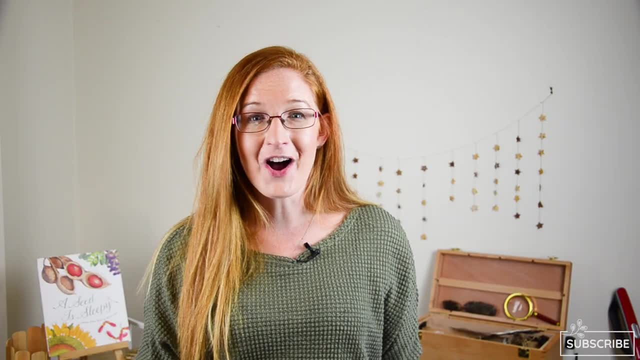 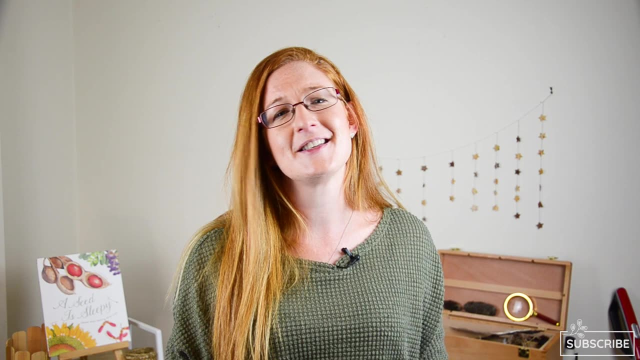 Number four: character nature crafts. If your child is enthusiastic about a certain character right now- whether it be a Disney princess or a talking tank engine, or maybe it's just a sweet teddy bear on TV- then this craft may be a real hit. You're going to have to get a little. 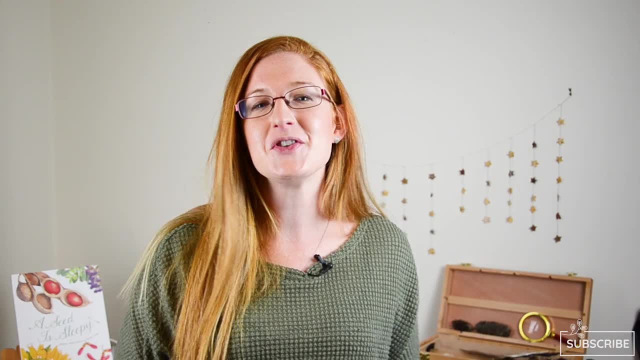 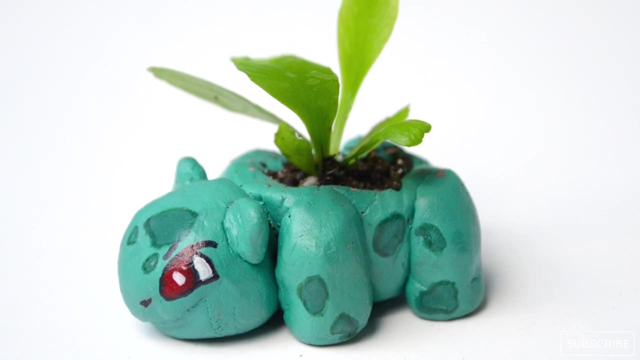 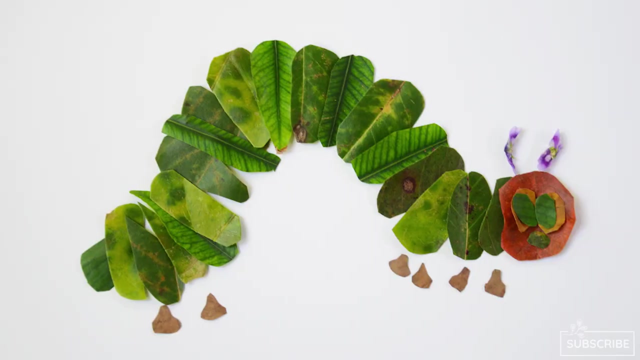 creative to set it up though. So here are some examples. If you and your children are openly or secretly Pokemon mad, I'm sure you'll enjoy them unplugging to get a little hands on by making these nature inspired Pokemon crafts. Or perhaps their favorite book right now is. 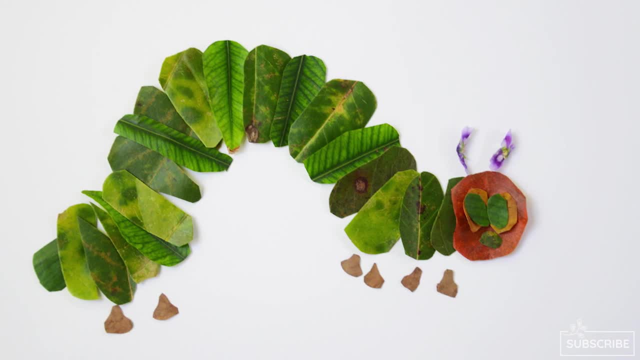 The Very Hungry Caterpillar by Eric Carle, in which case they can enjoy making a naturally created Hungry Caterpillar. So if you're interested in making a naturally created Hungry Caterpillar, make sure to check out the link in the description below and I'll see you in the next video. 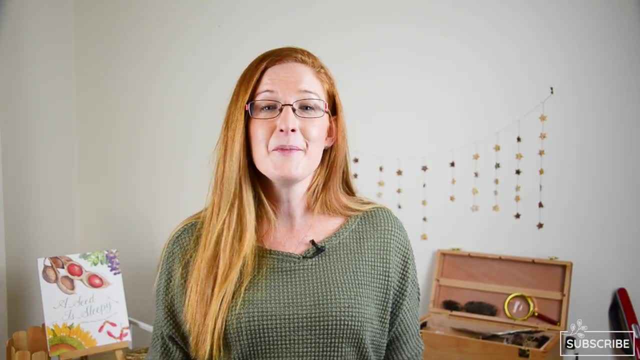 And if you're interested in making a naturally created Hungry Caterpillar, make sure to check out the link in the description below and I'll see you in the next video, Number five, weaving a basket with natural materials. Your child may struggle with this. 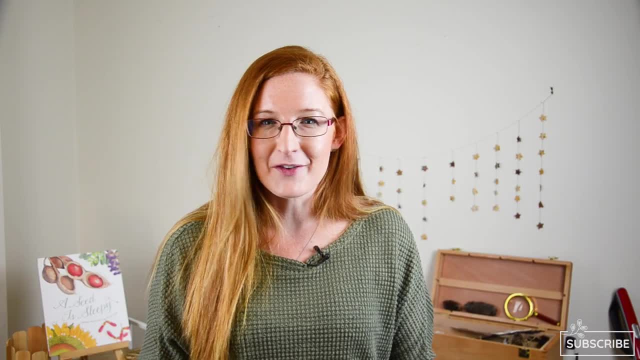 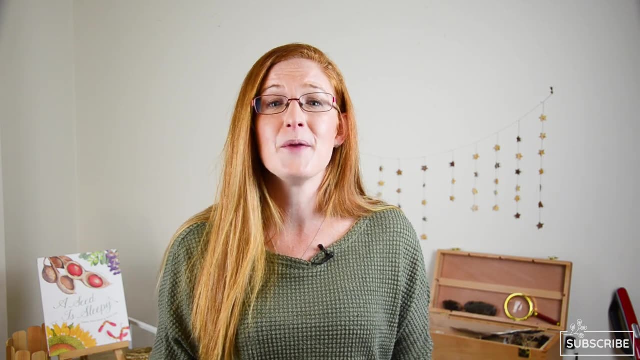 activity to start off, but that's all the more reason to give it a go. Weaving with nature develops a child's fine motor skills, and once they master this process, they too will learn that perseverance pays off. Don't push them, though. Just let them try weaving a basket on. 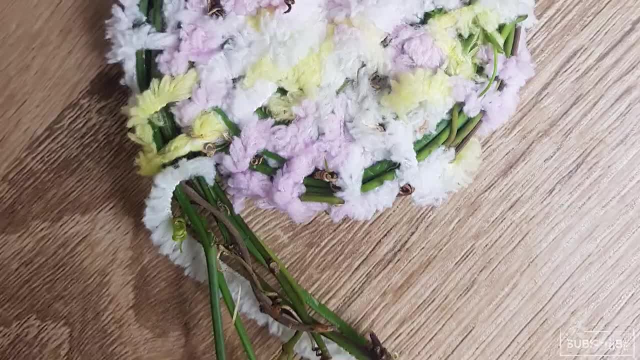 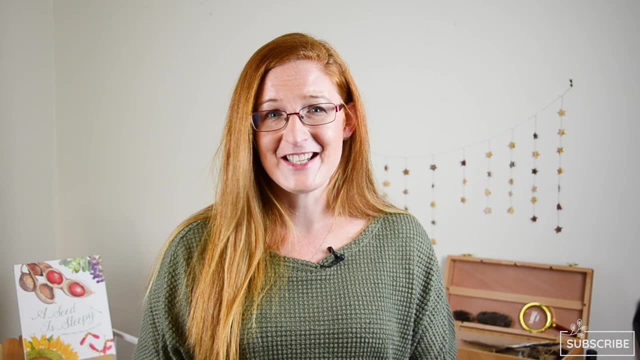 their own, and if they don't finish it, they can always try it another day. My girls will often get disengaged with the activity and then, when I'm making another basket again, they're out and they're ready to have another go. So get outside, collect some weeds and make your own, I'm sure. 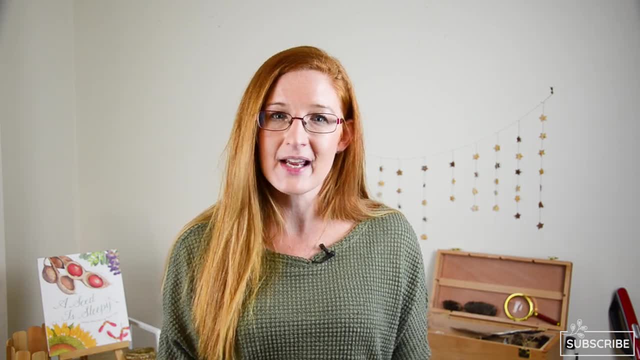 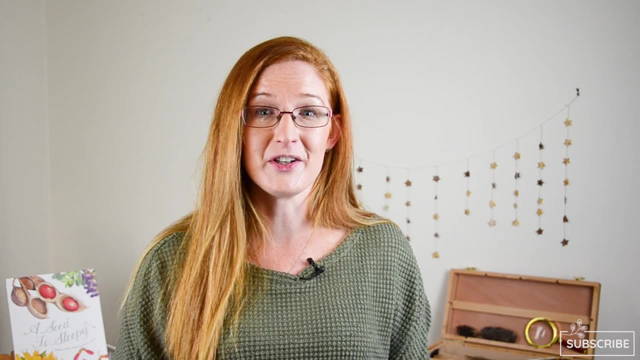 your kids will join you. It's such a beautiful time to reconnect with your child and celebrate the season. If you want to learn how to make a basket with natural materials, I've made a video tutorial on this for you. In fact, I've added links to all these crafts in the description. 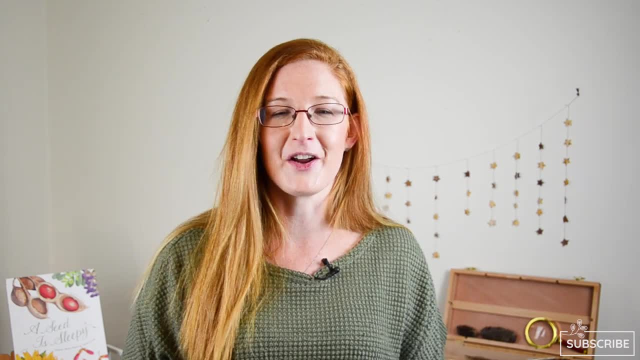 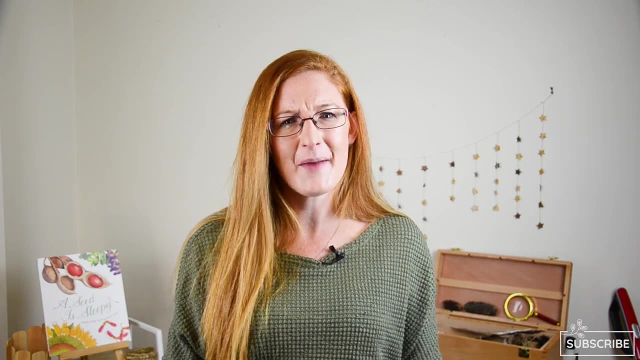 should you be looking for more inspiration or want to learn about a specific craft activity? If weaving a whole basket is a little overwhelming right now, but you still really would like to learn about weaving or show your children how to weave, then these nature weaving frames are really. 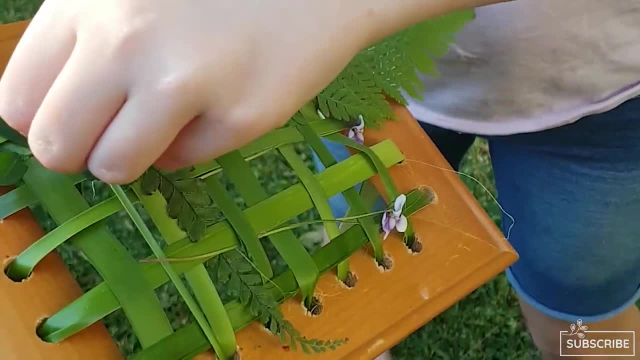 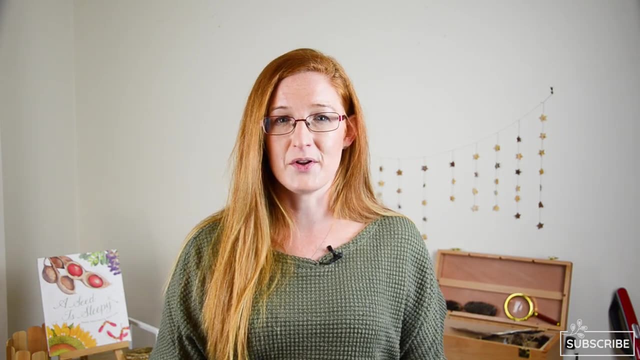 pretty and they're really easy to make, and you just use a recycled photo frame. So these are perfect for younger children and I'll make sure the link is in the description below for those as well. Number six: Earth Moss Ball. If your kids love messy play, they will adore this craft. Spagman Moss has this. 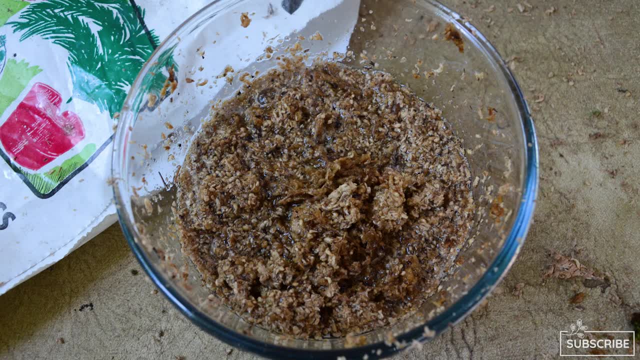 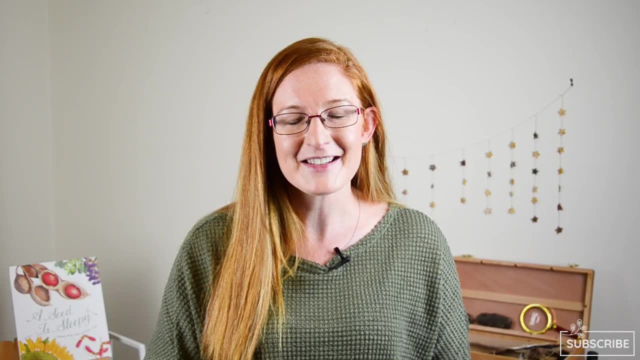 If your kids love messy play, they will adore this craft. Spagman Moss has this interesting texture and holds a heap of water, making it so much fun to play with. Kids especially enjoy wringing out the seaweed-like material and adding the moss on. So if your kids love messy play, 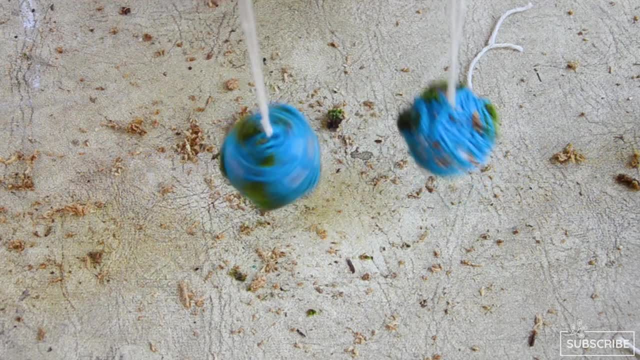 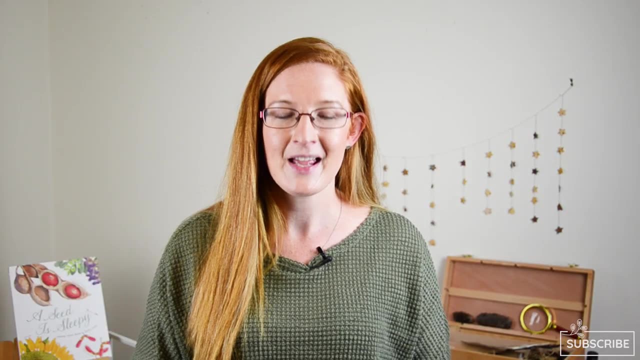 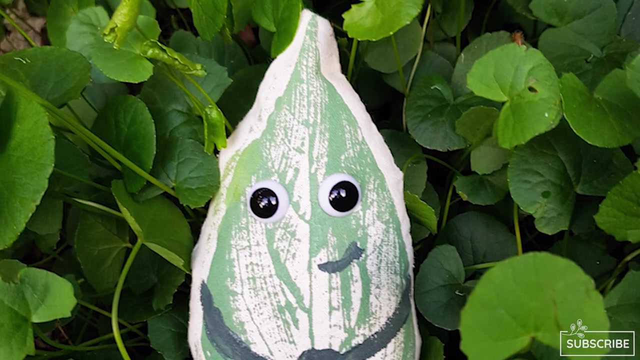 and want something to hang in their room and take care of. this is such a great nature craft for them and your kids will love spraying their moss ball each day to keep the moss lovely and green. Number seven: Leaf Softie Children are fascinated by leaves with all those different shapes, sizes. 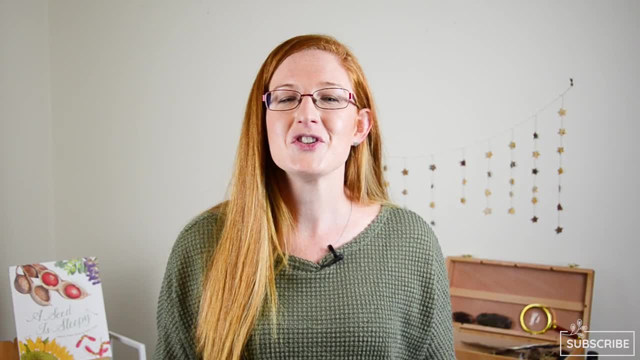 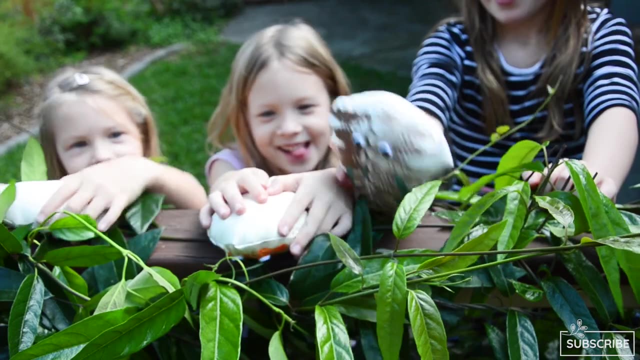 textures and colours. There's a lot to discover. If your child loves leaves, perhaps they would enjoy a homemade leaf toy to snuggle up to at night too. There is some sewing in this activity, so it's likely your child will need supervision, but that means you can join in the fun If you're. 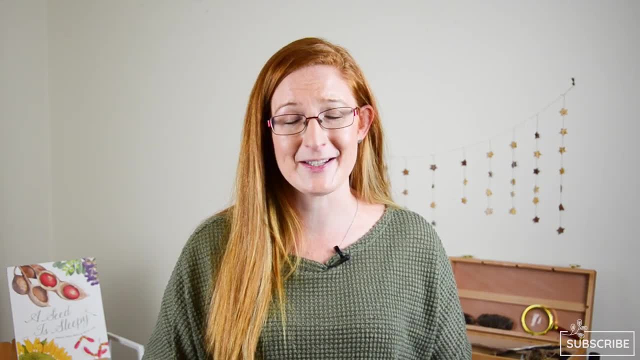 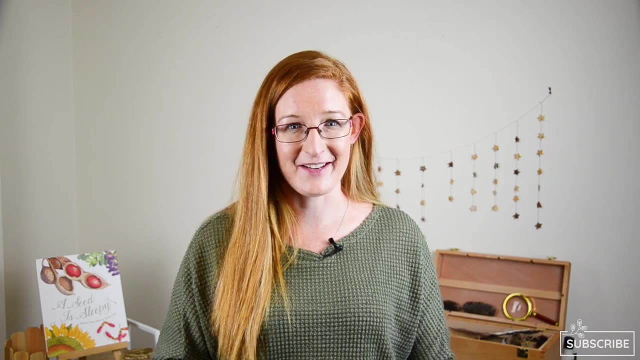 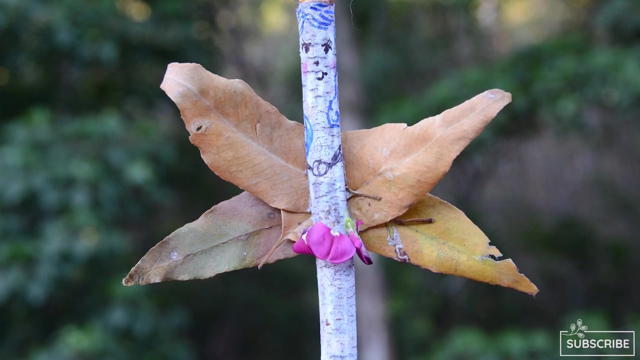 not a confident seamstress. rest assured that this project is very simple and completely hand-sewable. if you'd prefer to avoid the machine Number eight- Nature Fairy, I couldn't resist adding a Nature Fairy into the mix. They are so enchanting and so much fun to make. Creating these fairies is a 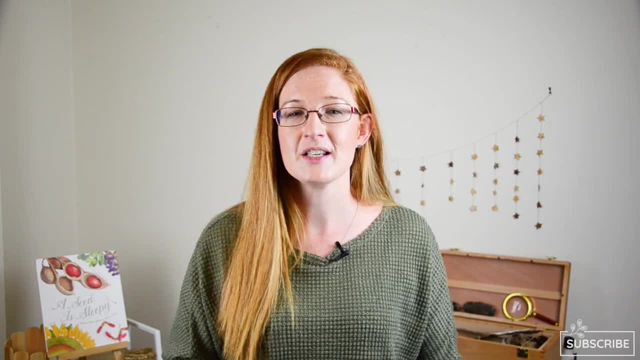 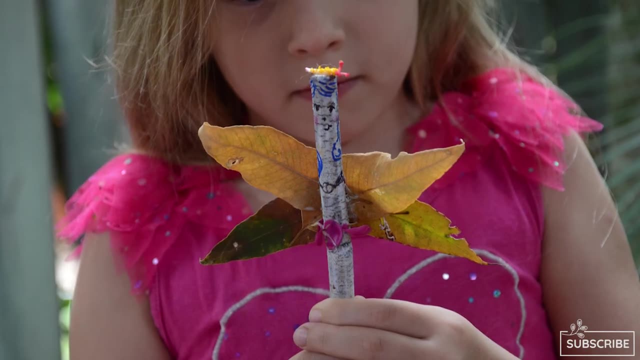 similar process to creating the butterfly craft I've already mentioned, but you might like to make them together so that your children will play with them. at the same time. We made three fairies, all uniquely beautiful, so make as many as you like. Number nine: Rock Painting. Now, I was late to the 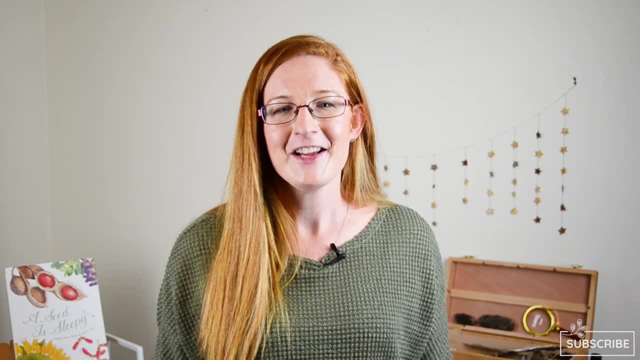 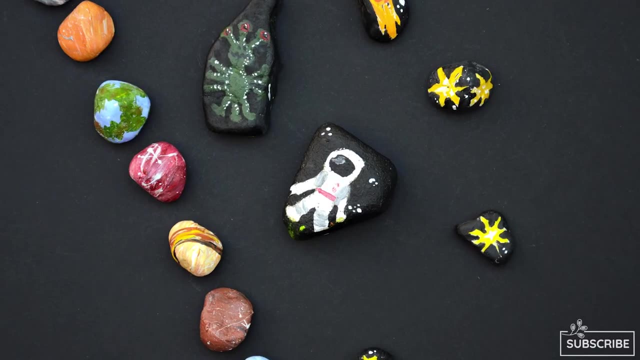 rock painting craze, but it's still really popular today. So set up a painting space outside and pull your garden and see if your child might like to get a little crafty. You could make these space rocks or flower rock puzzles. We don't waste our rocks. We paint on both sides, which makes them. 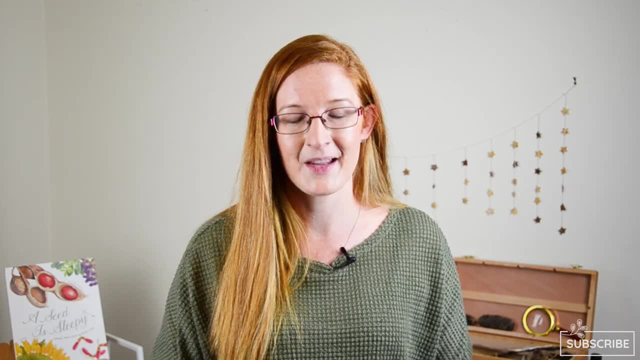 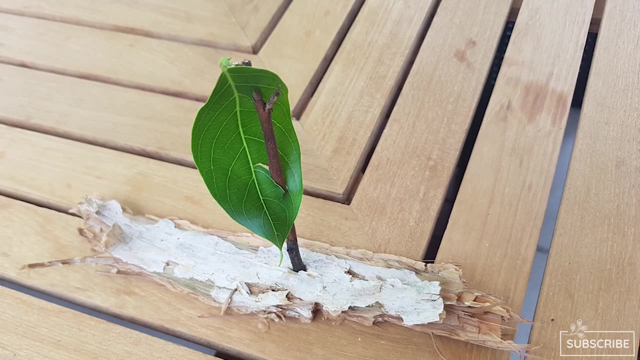 extra engaging and awesome for storytelling. Number ten: Nature Boats. Every child should make a nature boat and watch it float down a creek and easement or even in their backyard pool. It's a rite of passage and I'm sure you'd remember doing the same when you were a child yourself. 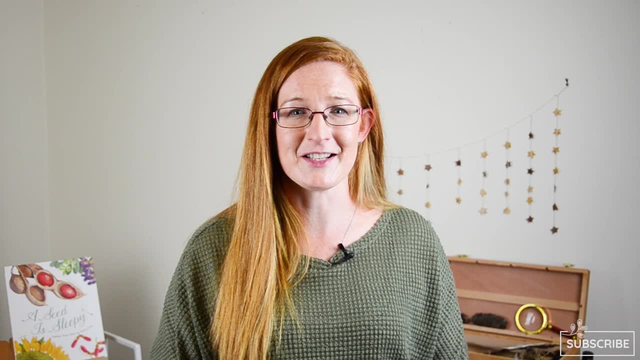 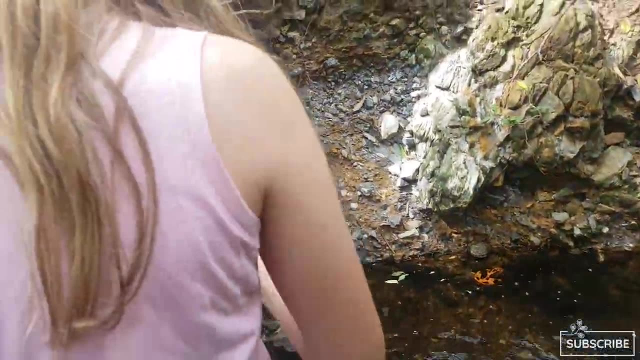 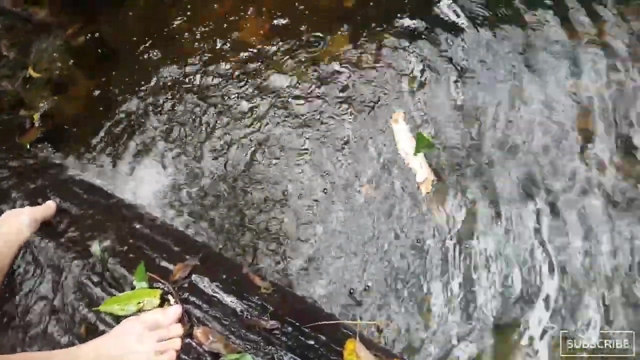 Nature. boats build fine motor development and promote problem-solving skills. Children feel a sense of accomplishment when they make something with their hands, especially considering that it must meet certain requirements to work properly. Every child remembers the moment that their boat, even after multiple trials, finally floats.